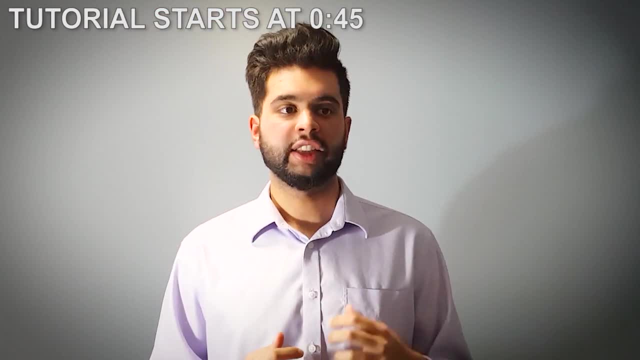 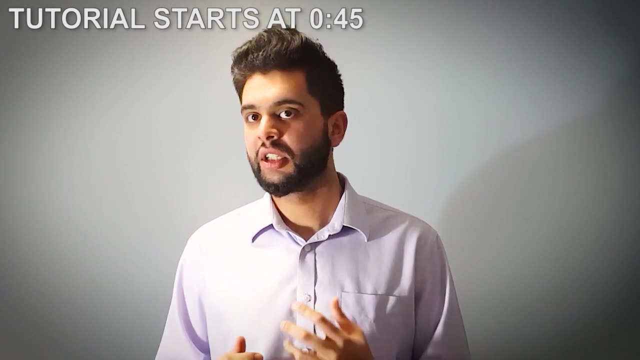 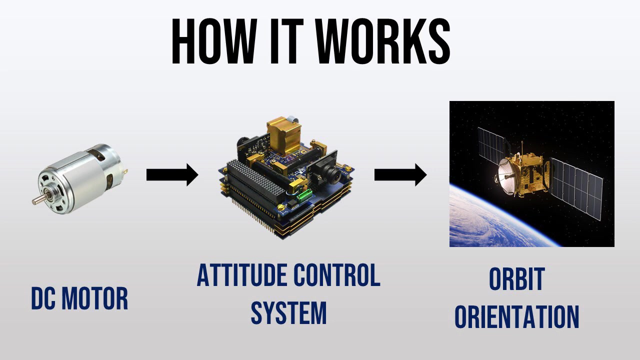 phone communications to talk to people on the internet and spacecraft must point a certain way when they orbit the earth because they must be able to transmit data with their sensors. So an attitude control system is simply a device placed inside a spacecraft which helps it orient a certain direction in the yaw pitch and roll axis. We'll be using a DC motor model which 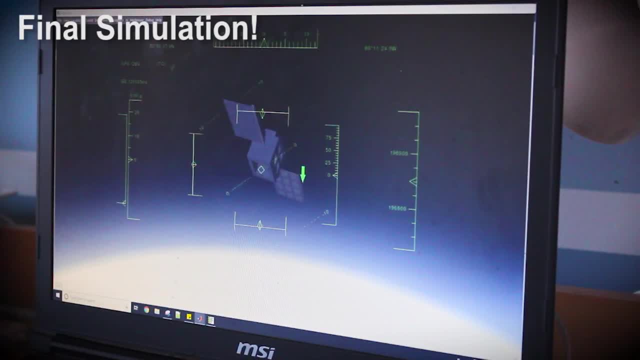 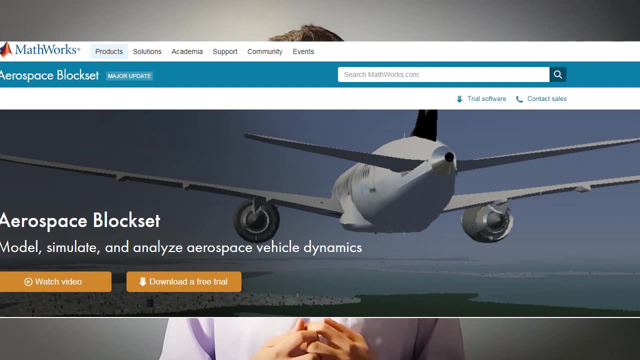 controls an attitude control system which will then rotate the spacecraft to point a certain direction. If you have never used MATLAB and Simulink, these are software which are commonly used in the aerospace industry by almost every single company out there because they make things very robust. 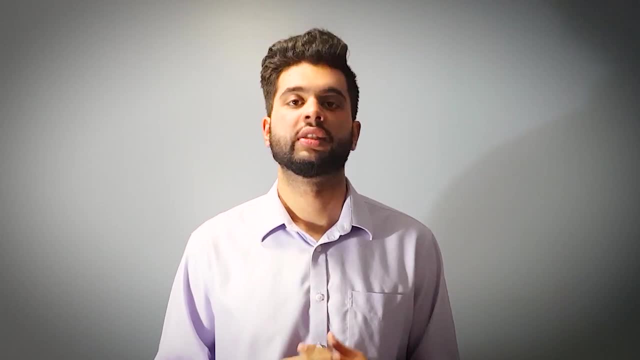 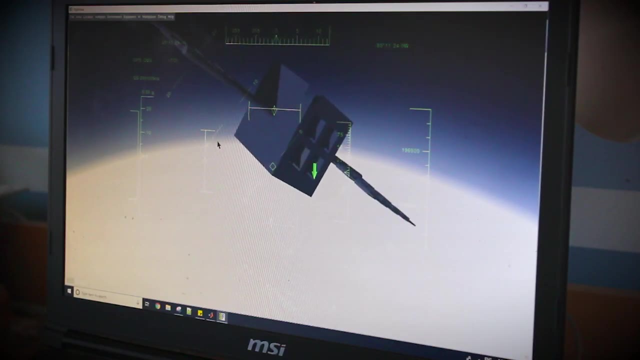 to solve especially for control system applications. This video will cover a step-by-step tutorial of MATLAB and Simulink along with FlightGear which is an open source simulator and I'll be showing you guys in a very detailed process how you can do this yourself. Let's get started. 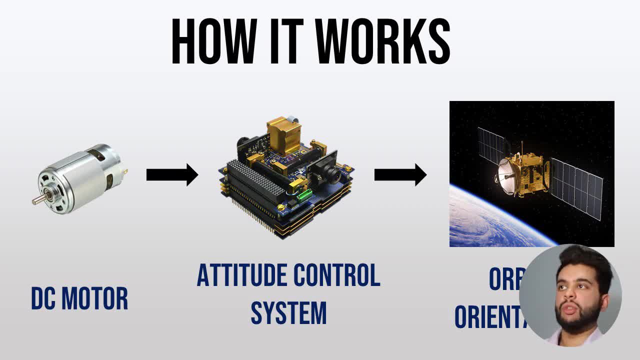 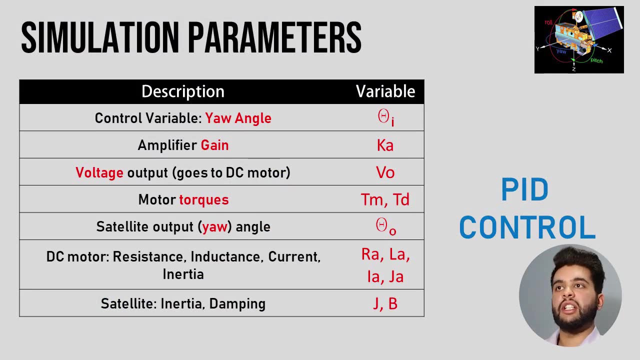 Okay guys so here we have the problem. We simply have a DC motor which controls the spacecraft attitude control system and that will orient the spacecraft to its desired yaw angle which we will input ourselves. The control variable which we want to control ourselves is the yaw angle. We'll be using a PID controller because that's a very commonly used tool in industry. We have an amplifier again to you know maximize the signal. The DC motor makes the voltage output but we will also need a voltage output from our circuit and the motor produces a torque which is TM and TD. TD is a disturbance torque which comes from things like noise in the system. 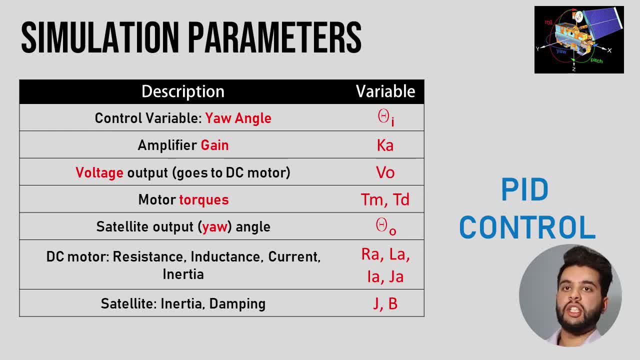 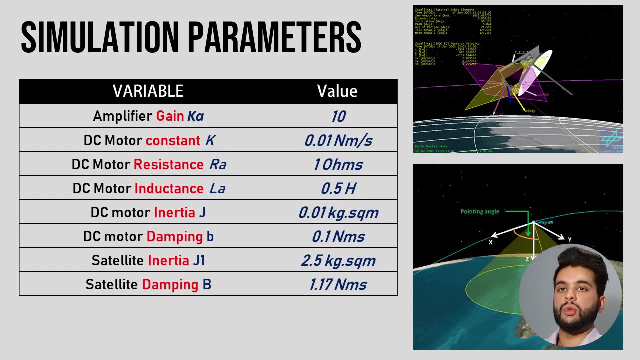 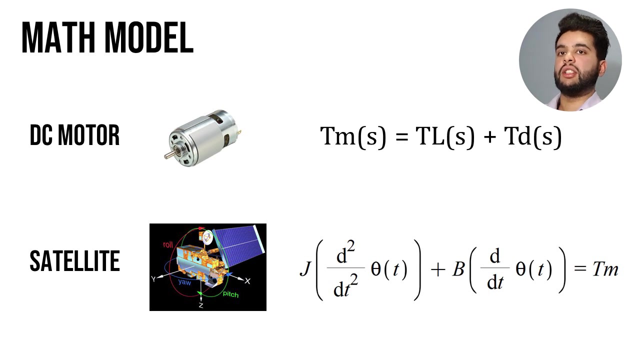 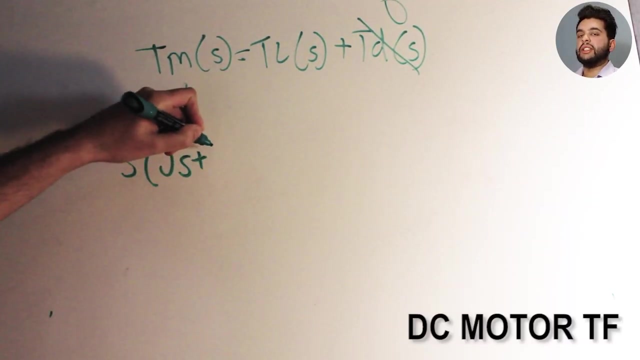 The DC motor will be a circuit as you all know in electronics engineering and circuits have you know things like resistance parameters inductance and stuff like that. So the motor circuit will have the following RA, LA, IA and JA. The satellite itself is a rigid body which means that it'll have a moment of inertia and damping as well. Damping can be set to zero but we will use it for more realism. And here are the constants which we will use. Now this will change depending on your problem but for this example I'll be using these values here. So let's see what happens here. And everything is in SI units. So the math model is the DC motor there and the satellite here. So these are the governing equations. Now this can be found anywhere on the internet and from here we can derive the transfer functions. You can see me doing the DC motor here. 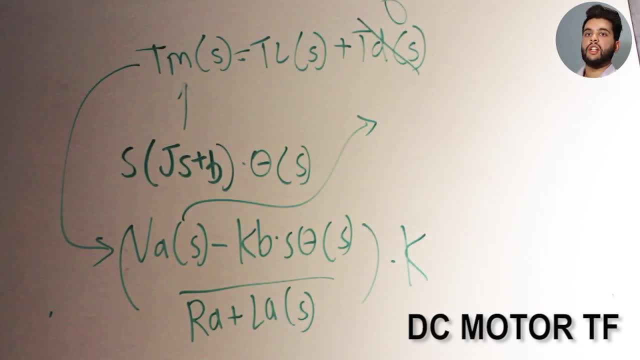 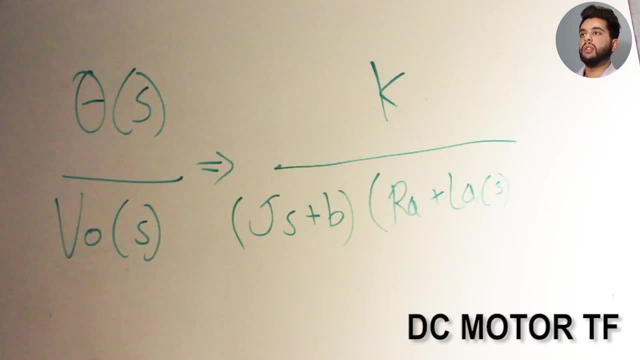 You simply take a Laplace transform and move things around to get the transfer function and for the satellite itself you get the exact same thing. For the satellite it's a lot easier because it's a Laplace of the equation and then you get 1 over j s squared plus b s. 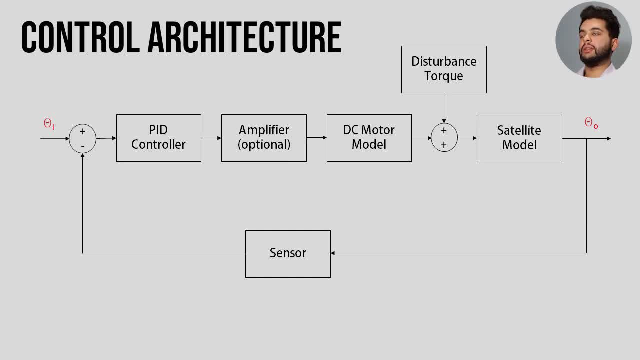 The control architecture is here in Simulink and Simulink is a tool used to design these things very quickly because we can use Blount diagram location. We have the controller, the amplifier, the motor and the torque which is going to the satellite model and then we have a sensor for feedback because this is a feedback control system and we want it to be a closed loop system so it stays stable and does not diverge. 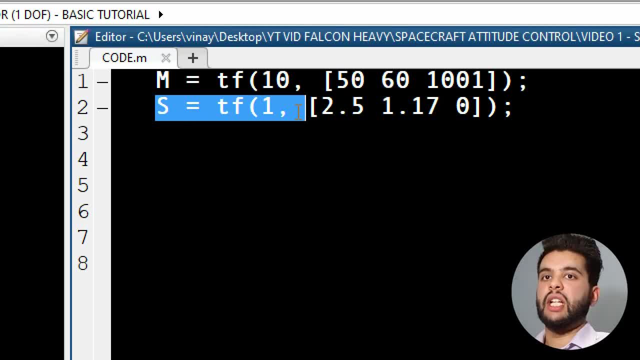 So if you guys open MATLAB we can now do a stability analysis of the system. 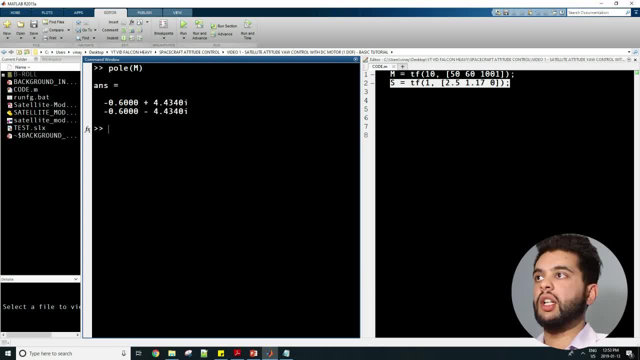 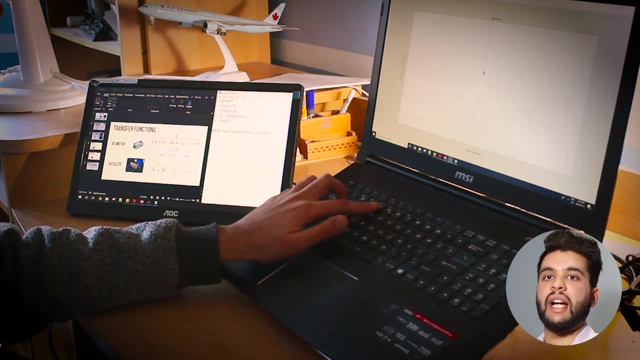 So if we first look at the motor which is m the transfer function for the motor. So we simply first find the poles by typing in pole m and if they both are negative which means that we are in stable region so that's good. Next we can plot a root locus. So a root locus is something which we can use to determine where our system lies in the xy plane. We want everything to be on the negative side. 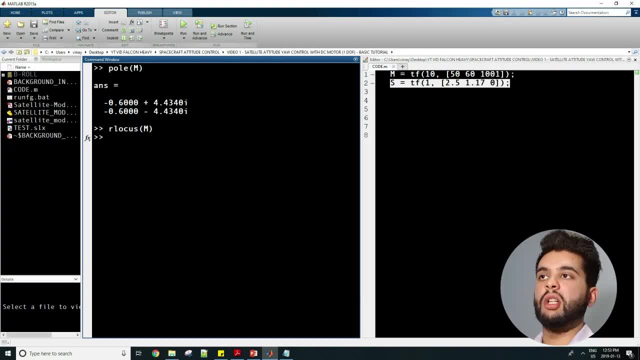 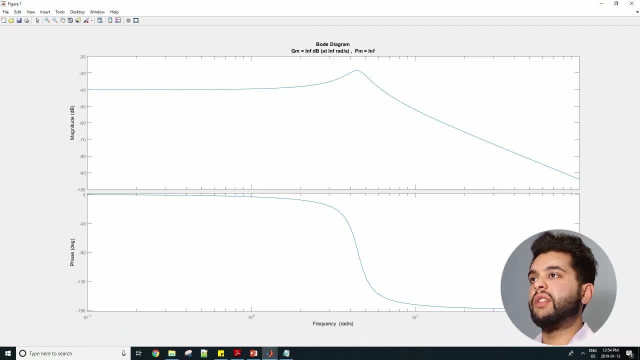 Next we can do a gain and a phase margin. This is called the Bode plot as you all know in control systems and this plot we can you know look at it at different frequencies and see what we have. So the frequency and the magnitude will change out of this different value and this is quite common right like no system will stay stable at every single operating frequency. 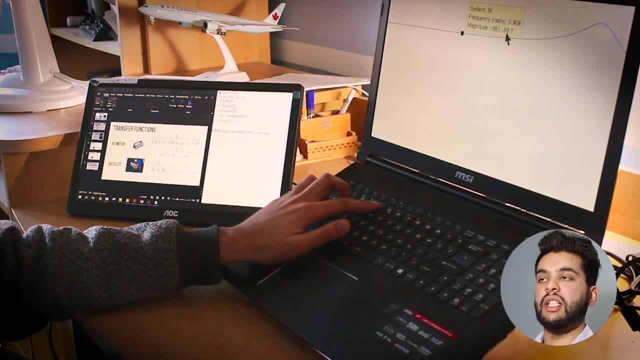 At some it'll be over damped, at some it'll be under damped, at some will be critically damped. 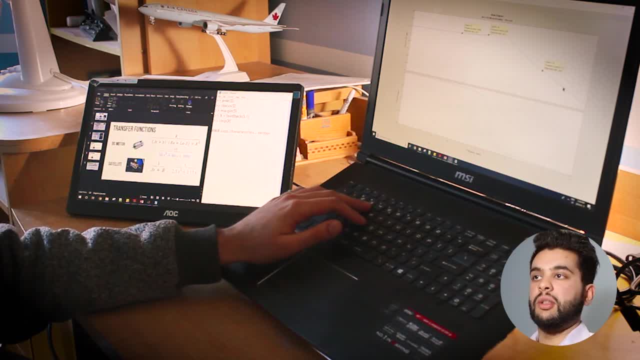 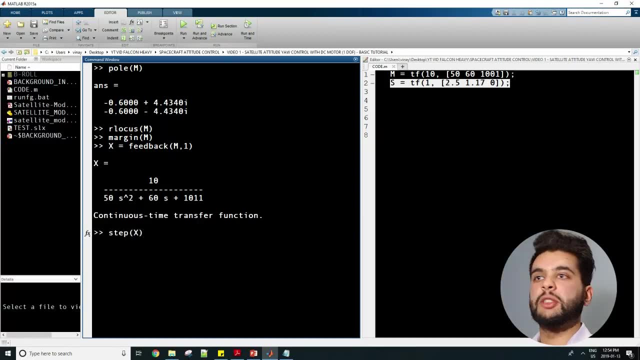 So we must look at this behavior as we go along the frequency spectrum. Next we can do a feedback loop and to look at a step response. So a step response is simply a unit input or it can be something else but in this case is using 0.01 as our unit input. 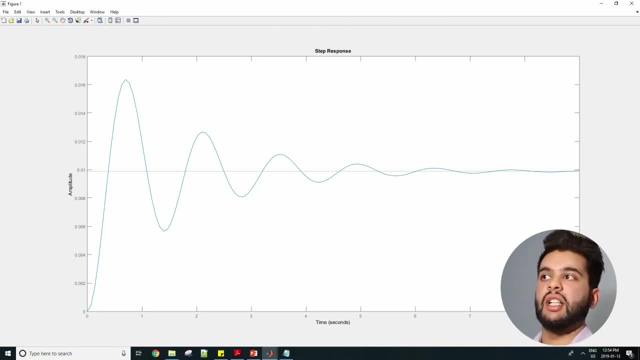 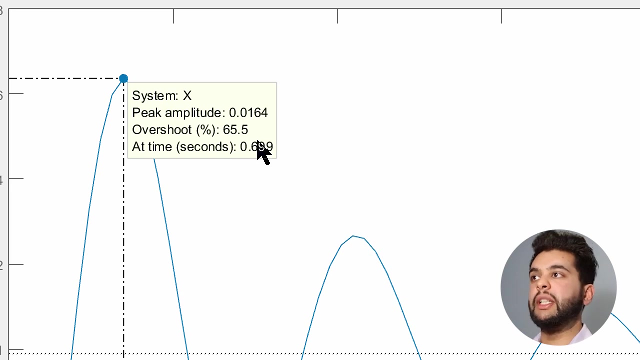 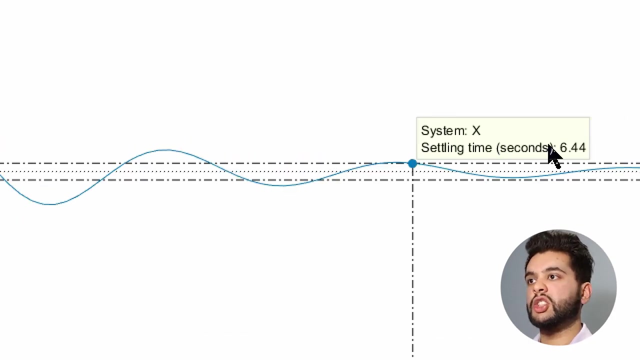 We do have some oscillations there in our system of the motor but this is because you know we don't have a controller yet right it's only the feedback unit feedback. So we do have quite a big overshoot of about 65 percent so you simply right click on the graph and select peak frequency and you'll see that it's a bit higher. Next we can look at the peak response to get that. So our goal is to minimize that you know like 20 percent or something. We also have a decently high settling time of about six seconds. Now for the motor it's a very long time so we must reduce that. 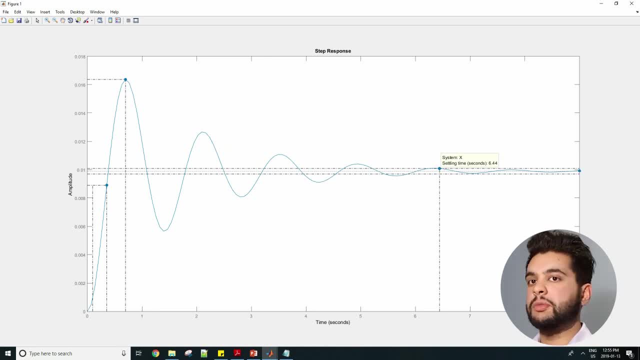 Next we also have rise time. So the system does respond very quickly in less than one second which is a good thing right and our steady state value after about nine seconds is about less than one percent which is a good thing. 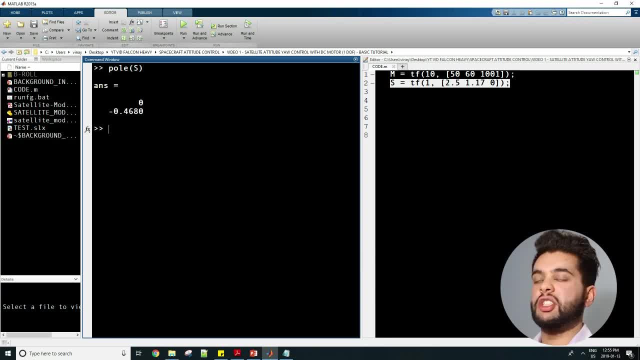 Next we can look at the satellite model. So this system is marginally stable because we have a zero there and if it lies on the zero plane it means that it is marginally stable so it does have a potential to become unstable after. 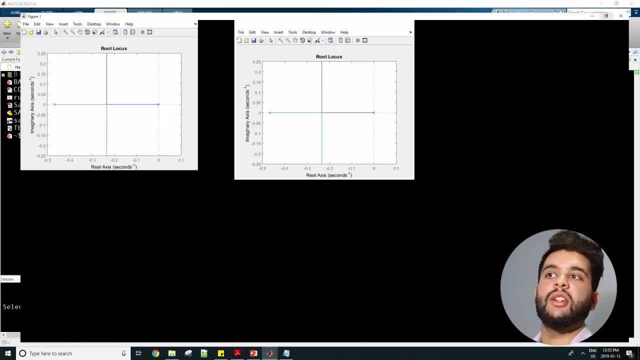 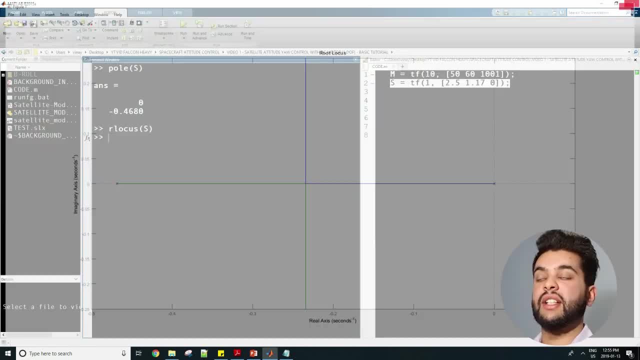 If you look at the root locus we can confirm this we have one point lying on the zero zero point in the xy graph so it tells you that the system is marginally stable but we must converge towards the negative side as much as possible. Looking at the gain and the phase 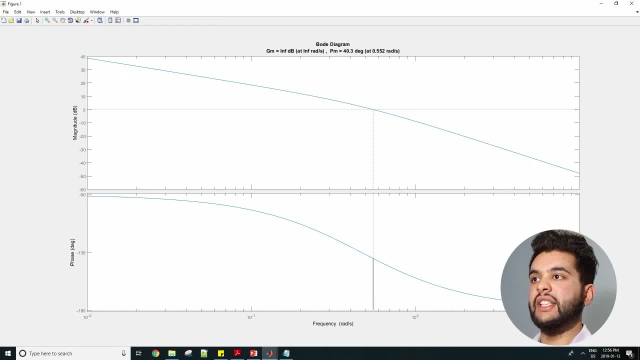 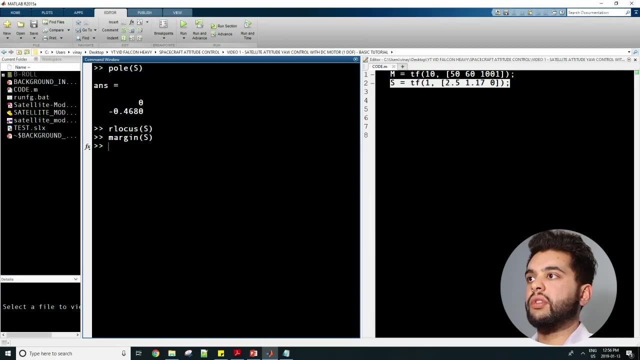 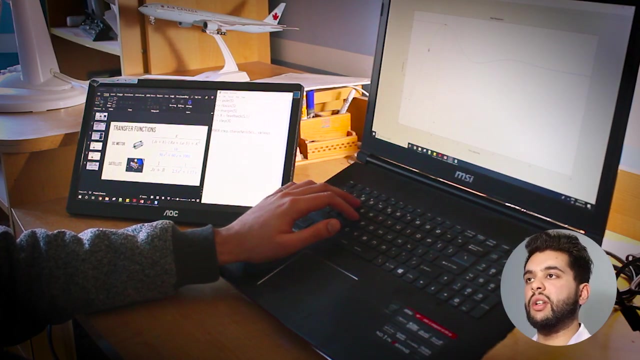 margin they're both decreasing so you know like it's not a very stable system so we must improve this as much as we can. Looking at a step response we can do a similar analysis it does not oscillate as much which is a good thing but it does have a very slow converging time right the overshoot is about 28 which is quite okay but we can also do better at that but it does have a very slow 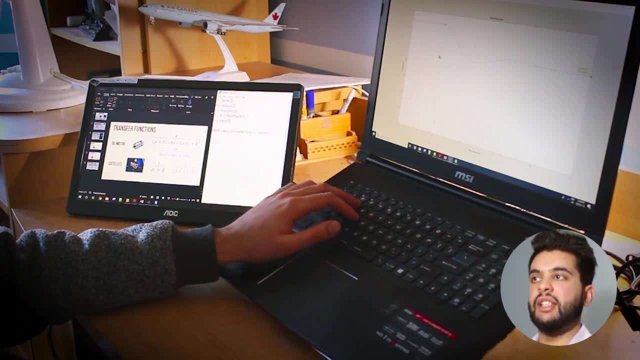 response. Now for satellites they don't you know spin very quickly right they spin quite slowly and you want the spacecraft structures to be safe and you don't want it spinning too fast it can cause damage to the sensors and stuff unless it's for a specific application in which you need it. So here 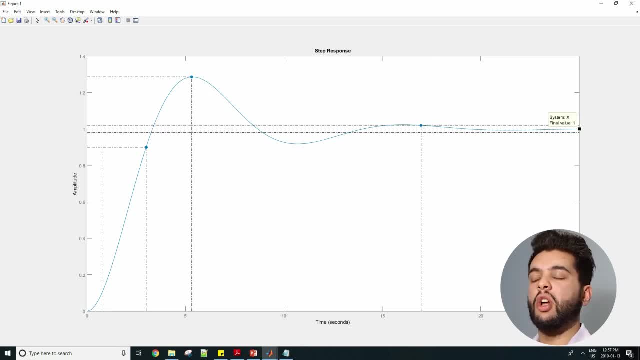 we have about a 17 second settling time which is a bit too long but you know I guess we can improve it by using a controller. 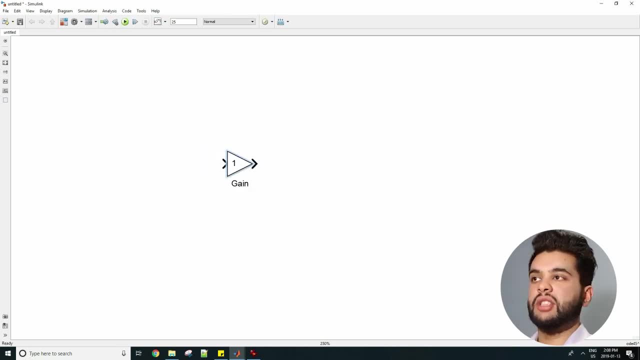 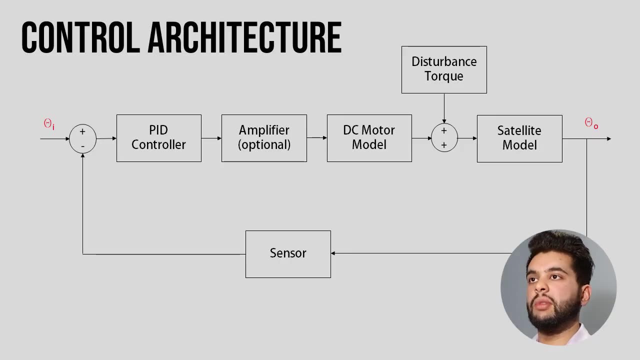 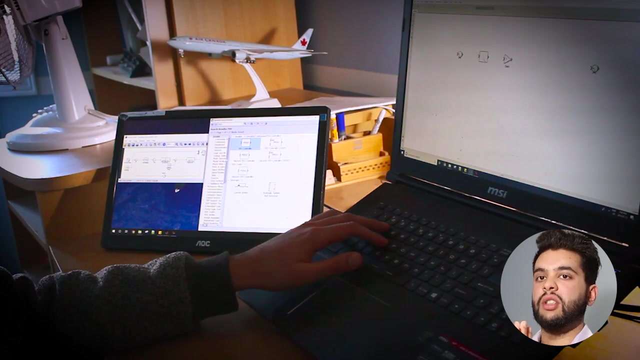 So now let's go to Simulink and drag in our blocks. So we simply use the control architecture and drag in blocks. You use the Simulink library browser and you can simply drag in constant you know block just drag in everything and set up your problem. Simulink uses block diagrams which makes things very easier and we can save a lot of time you know instead of programming everything by hand right. MATLAB does have programming tools by hand but it's a bit slower and Simulink you can change things very quickly and see how the system will respond to different inputs. 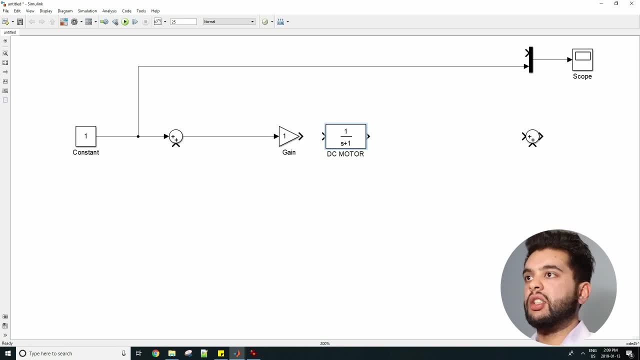 So I'm simply dragging and connecting everything. The transfer function of the motor we have 50, 60 and 1001. Because it goes by s square s and then one right. 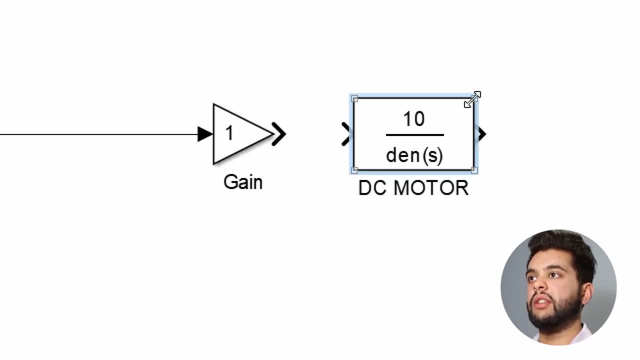 So we can simply you know make that show it there so do the same thing for the satellite as well. We can drag in a PID control block here and then change the parameters after. 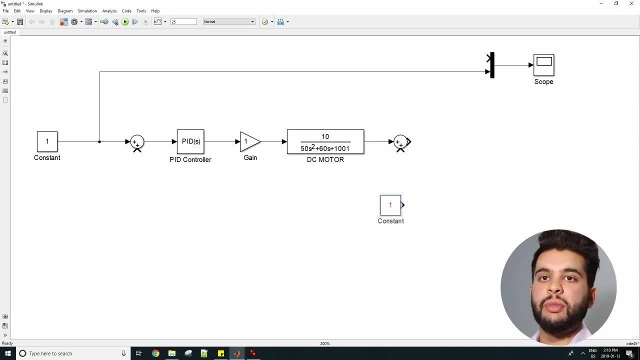 That's our disturbance torque or TD. Now I've set it to be constant here but in most applications the disturbance torque is a stochastic value which means that it changes with respect to the satellite model. And what they do is they do a stochastic analysis and they see based on the satellite's conditions what the torque will be. Now this is a very random process so there is no fixed value but for now I'm putting it constant. 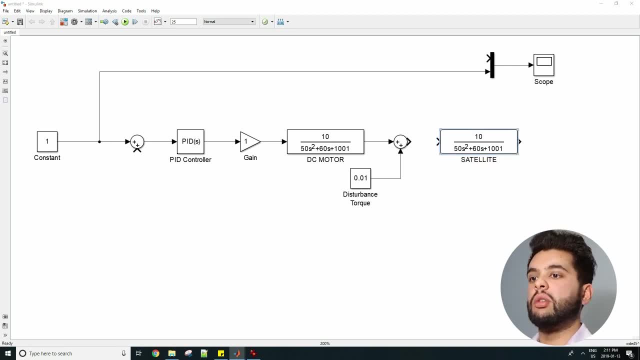 For the satellite use you know gs square plus bs so we'll be using 2.5, 1.17 and zero. 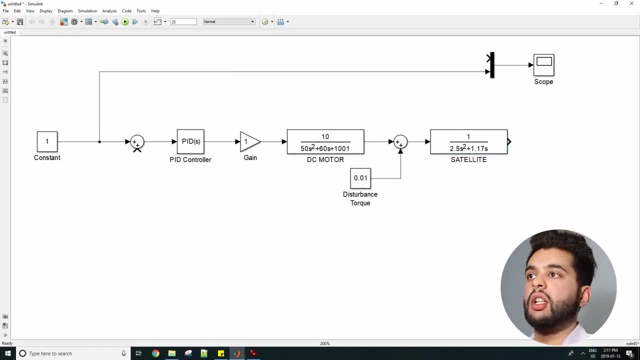 So just now connect the blocks and everything let's you know put our sensor in there of unit feedback which is equal to one for now. 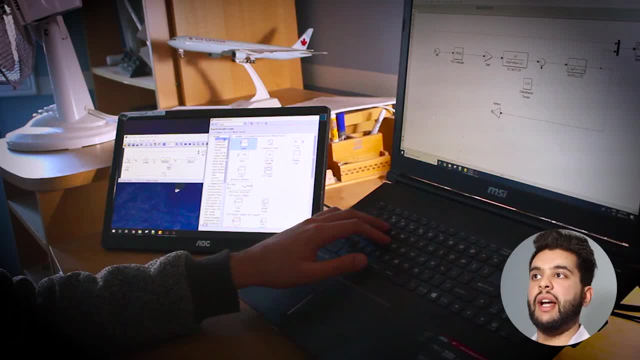 And click ctrl r to rotate. Block and then connect it to your negative feedback. So that's our feedback loop here. We now have a closed loop system. 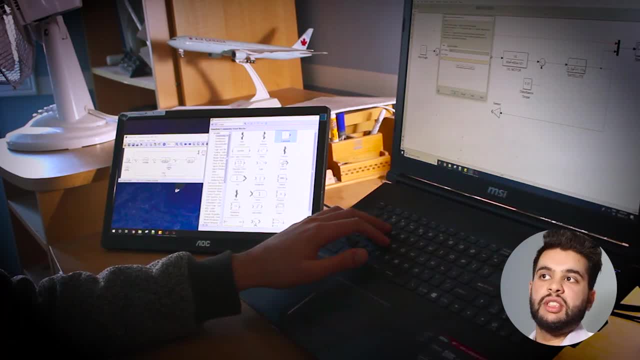 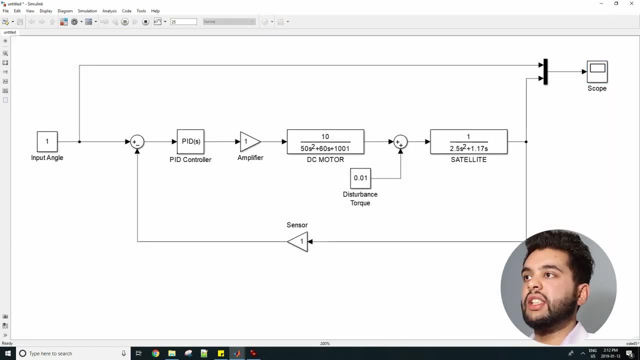 If you run this by itself we see that the system is diverging which is not good because obviously the feedback loop has not been connected yet. But when we connect it we still see it diverging but it is converging a little bit. So now let's tune the controller. 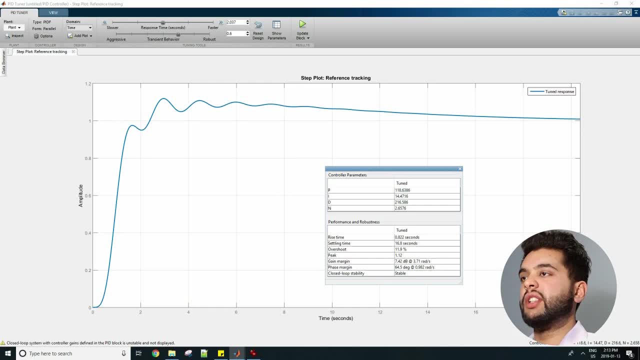 So linearize the planet and let's you know tune it. So when you this is our response here when you press tune. 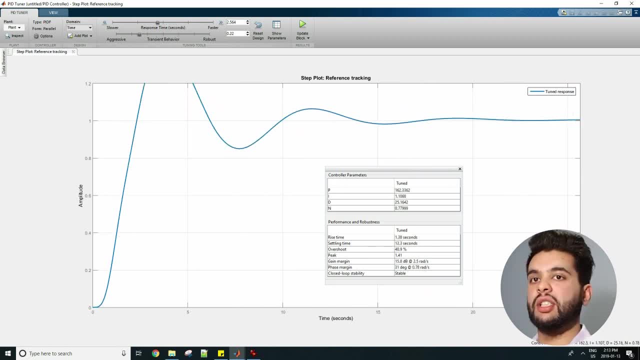 We can change these parameters ourselves to go in the top and you know drag in the stuff. 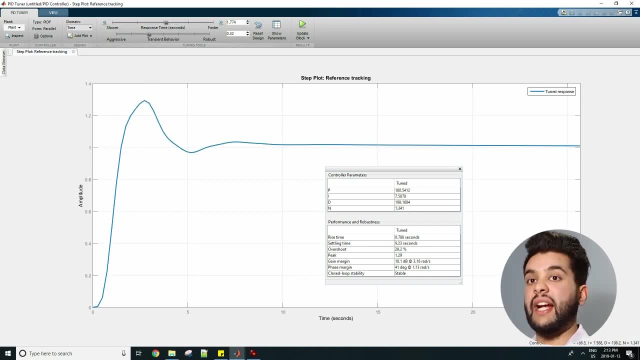 I've done another video showing how to tune a prd controller for a cascaded control system which is a lot more complex so I do recommend you watch that as well 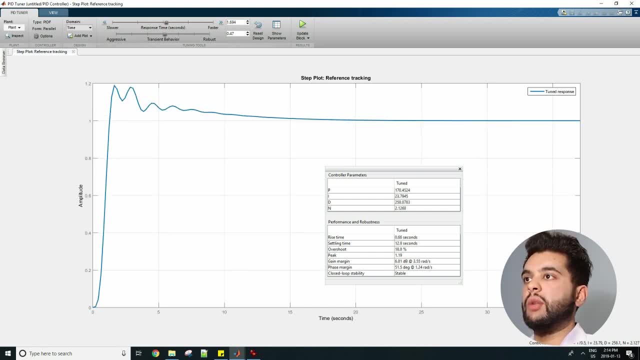 So just keep dragging in your stuff until you get something decent and when you're done our final response is something like this but we can always tune it. We don't want any oscillations you know 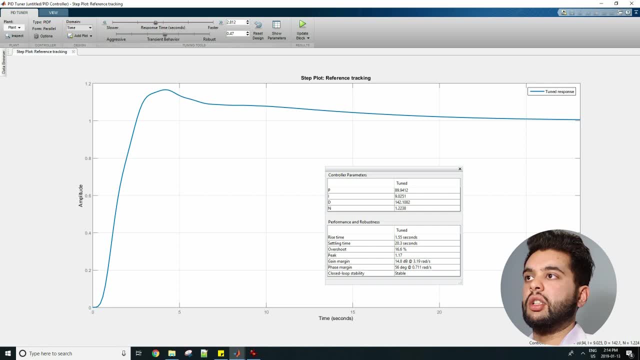 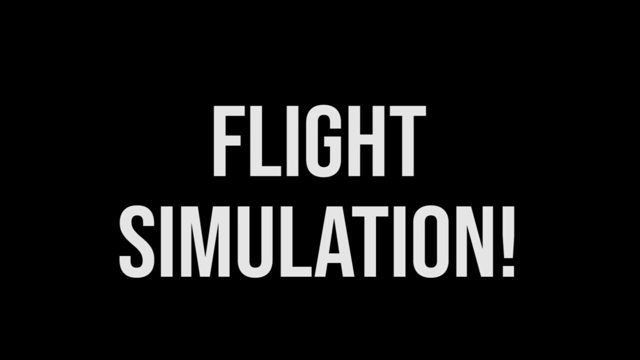 we want the system to converge safely. So we're going to turn this off and then we're going to do a converted demo. Let's see if we can do this. So that's our response and let's now go into flight gear and see what it looks like. 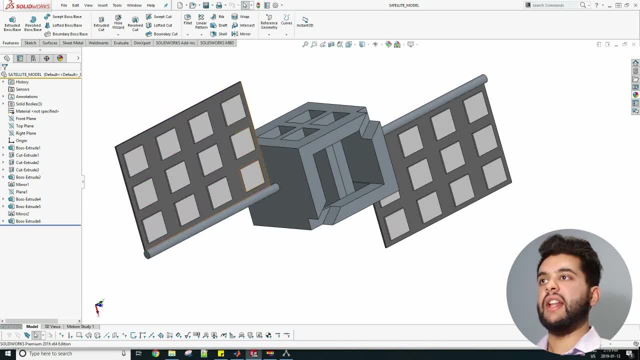 Okay guys so I did make a satellite model in SOLIDWORKS so you can use any CAD software for